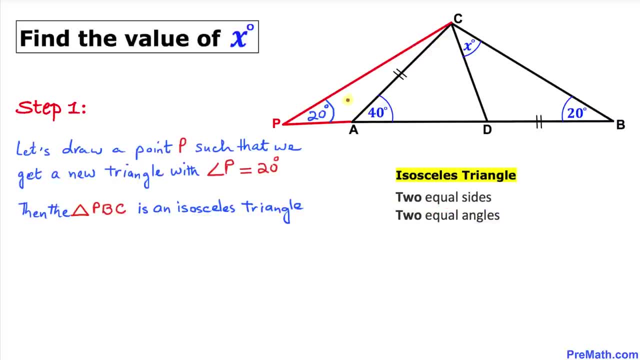 So thus this triangle, PBC, is an isosceles triangle because this angle equal to this angle and according to this definition, then this side PC is going to be equal to this side BC. Thus we got PC equal to BC, And now let's recall this exterior angle theorem. 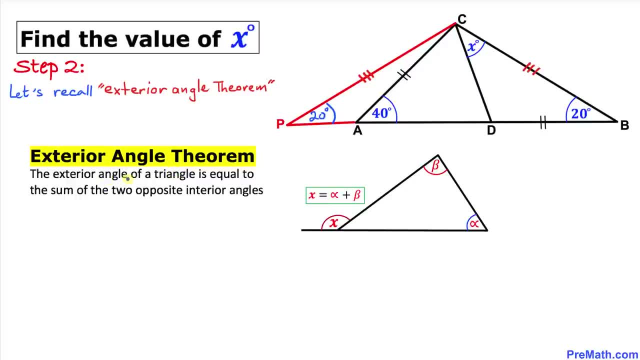 And here's our exterior angle theorem. The exterior angle of a triangle is equal to the sum of two opposite interior angles, as you can see in this example, And here, in this case, X is our exterior angle and alpha and beta are our two opposite interior angles. 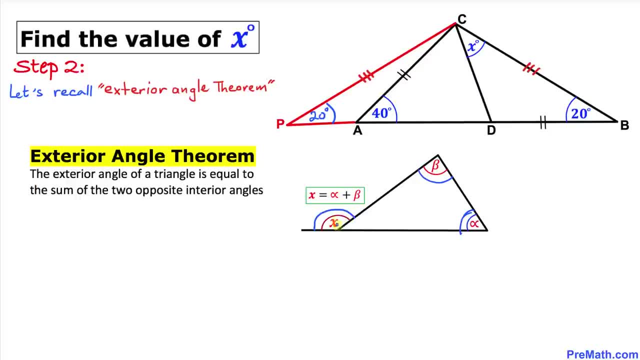 Then, according to this exterior angle theorem, this exterior angle is equal to the sum, the addition of these two opposite interior angles and in our case, this angle a is going to be our exterior angle and this angle p, and then this angle p, c, a are our opposite interior angles. so therefore, this exterior angle, which is 40, 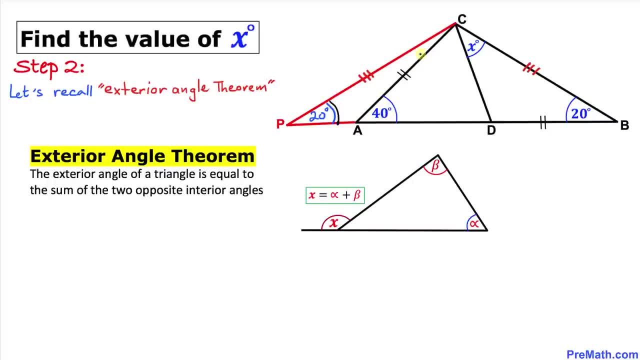 degrees is got to be the sum of this angle plus this angle. if this is 20 degree, then this angle is going to be 20 degree as well. so therefore, our angle pc, it turns out to be 20 degrees. so therefore, this triangle, pc, is an isosceles triangle, since these two angle this angle. 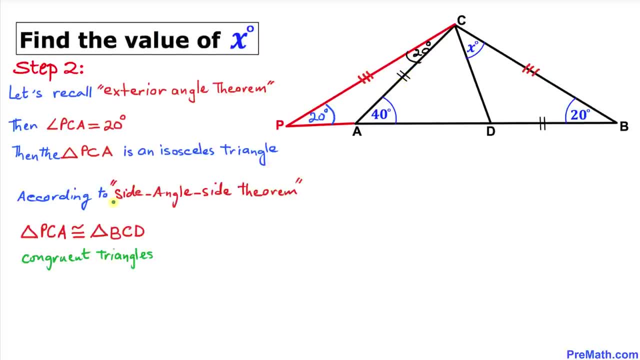 and this angle are equal, then according to side angle side theorem, this triangle p, c, a and the other triangle, b, c, d, are congruent triangles, as you can see over here, these two sides and the angle between them and these two sides and the angle between them. so thus, in these two shaded congruent triangles, we know that this side corresponds.